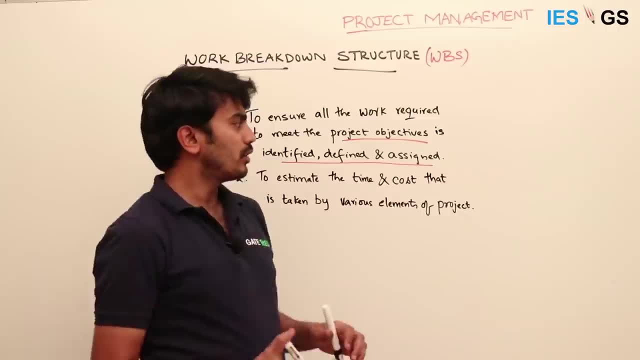 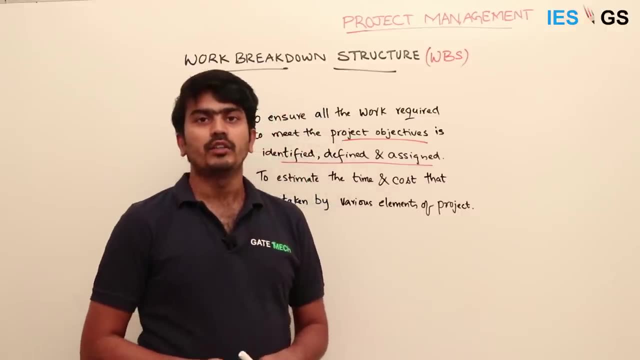 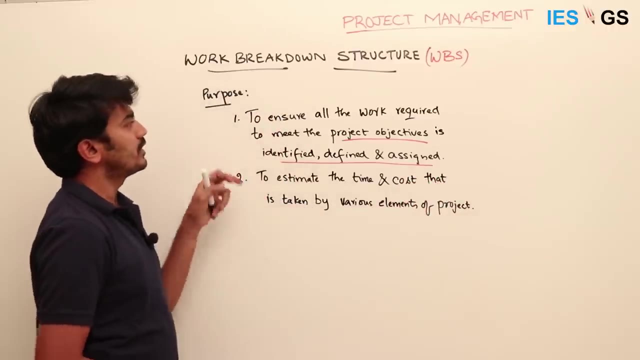 are activities we are going to perform. so, once we know that we we don't want to miss some, some components of work, some components of the project, so without, without, without identifying the entire details. so so this first purpose is to ensure that all the work required is identified, so that the costing and 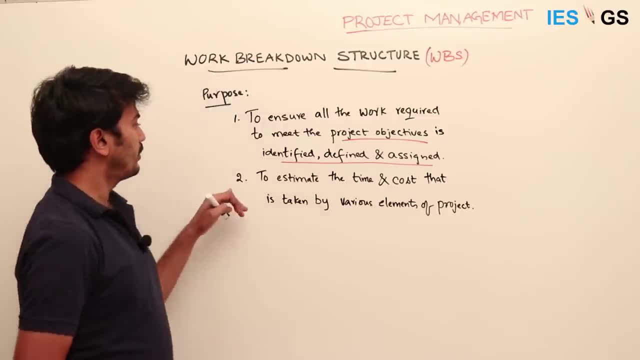 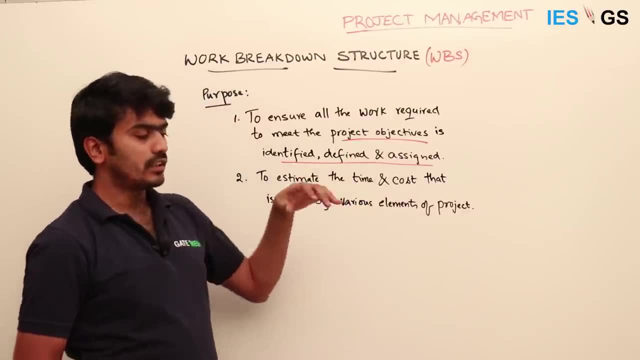 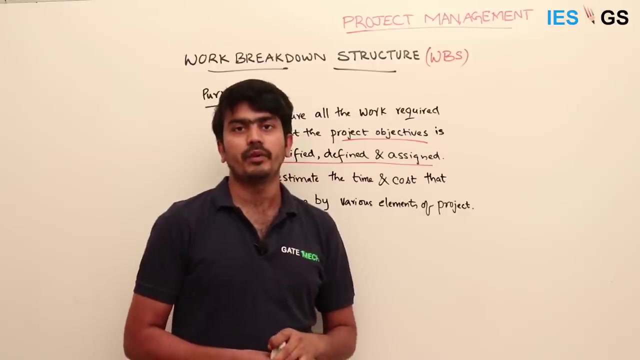 effort, the estimates will come correct, okay. and the second purpose is to estimate the time and cost of all these activities identified so that we will get the total project cost and the project effort timelines that are required. so this is the primary purpose of work breakdown structure. so, in order, 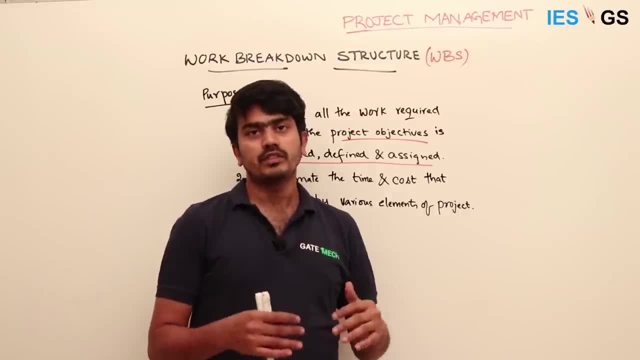 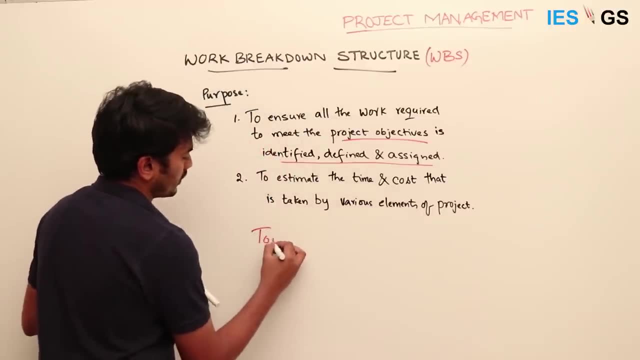 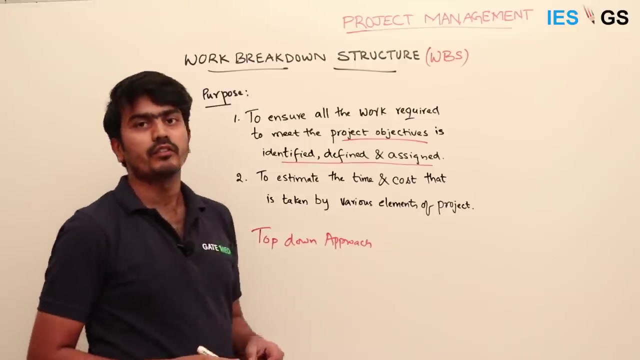 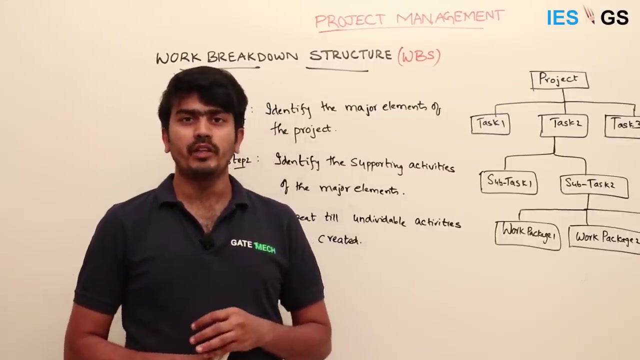 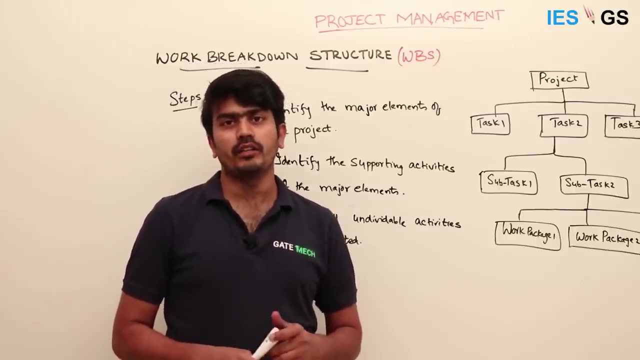 to construct this work breakdown structure, so we use some steps, so it is a top-down approach in order to arrive at, in order to arrive at the list of activities that we need to execute. this method establishes the logical framework for identifying the list of activities required for the project. so the main steps that are involved in determining a 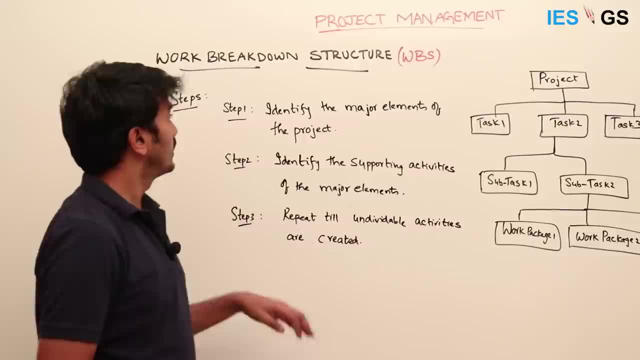 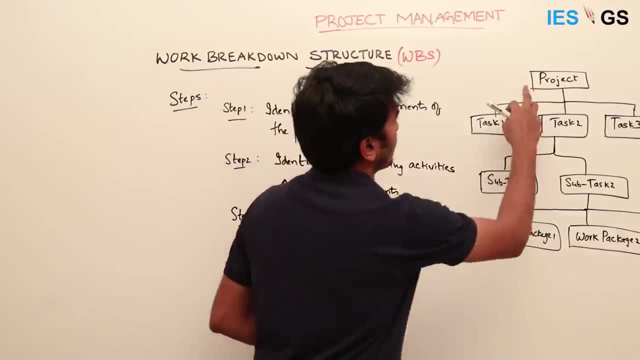 work breakdown structure from a project scope is like this: the first step is to identify all the elements of the project. so in this, in this picture, you can see the project is divided into three tasks: task 1, task 2, task 3. so when I say the major elements, 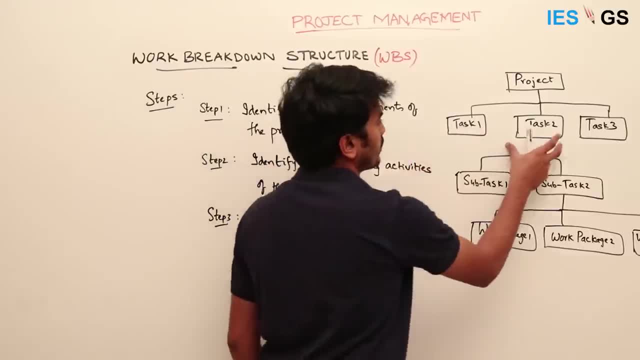 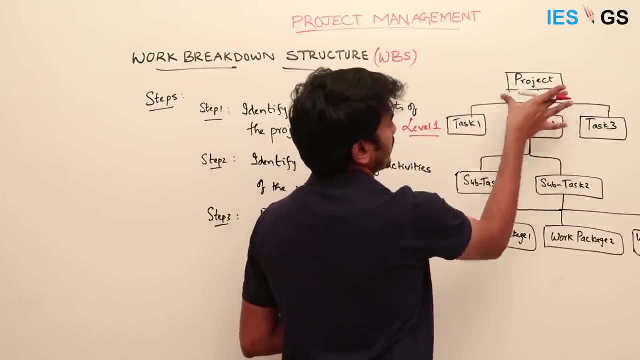 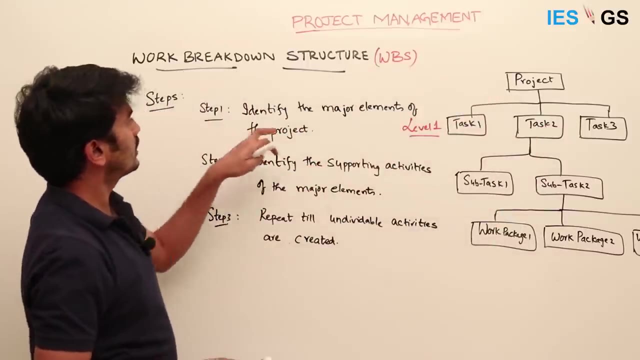 which define the project, which define this result: task 1, task 2, task 3, you call it, say level 1 in this level. so these three tasks form the project, these three, three tasks when combined and they form the final project. so once we have the major elements and then we break down this major elements again, task 1: 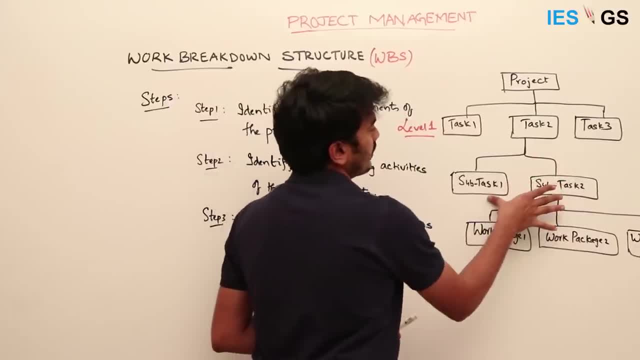 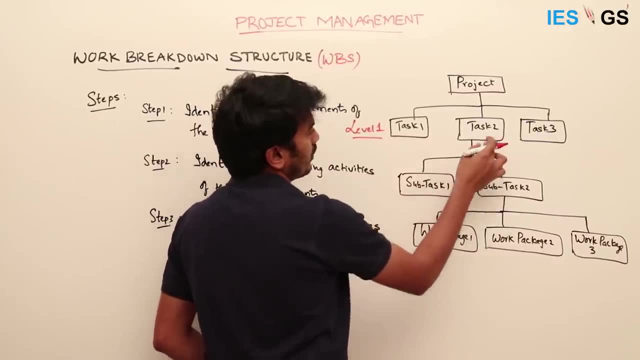 task 2 and task 3 into next level of items, our next level of activities. what does task 1 comprise of? what? all activities are there? what does task 2 comprise of? so here in this picture, I considered subtask 1 and task 2. 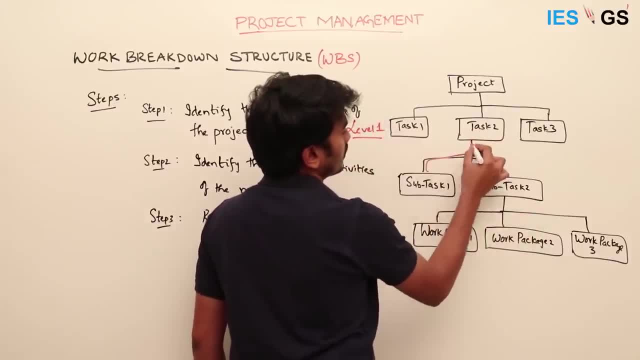 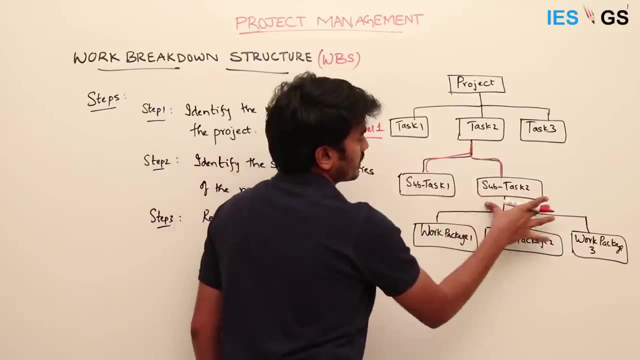 comprise of task 2. so this is the next major element which is which is consistent with task 1 and task 2. so this is the next major element which is consistent with task 2. so this is the next major element which is consistent: these two activities, subtask 1 and subtask 2, and again, subtask 2 forms three. 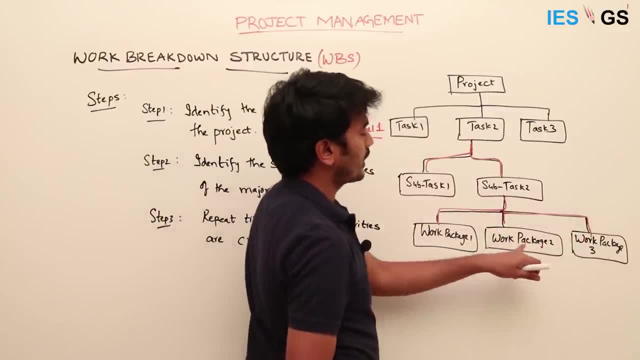 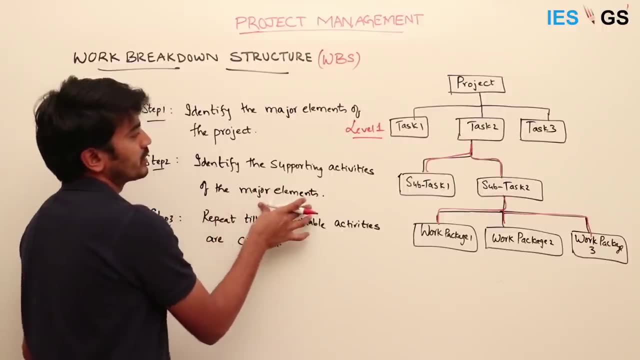 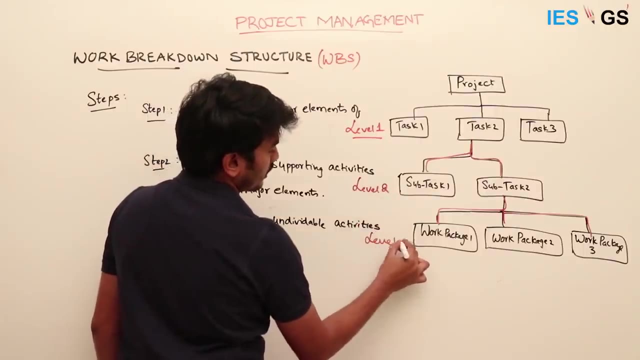 activities called work packages, work package 1, 2 & 3. so we are identifying, that is, a step 2, identifying the supporting activities of the major elements. these two are supporting activities of task 2 at level 2 and these are at level 3. work packages are at level 3, which supports the subtask 2. so 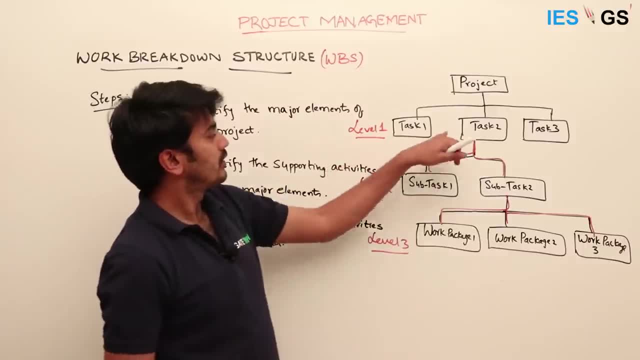 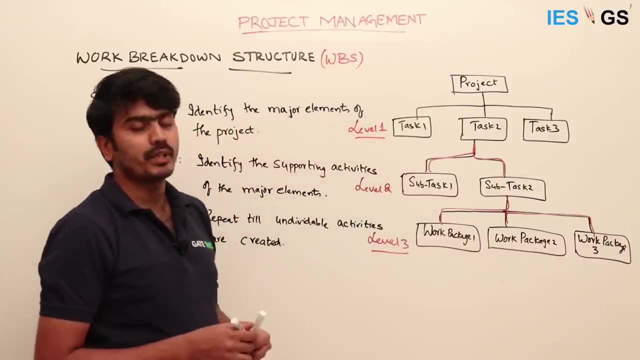 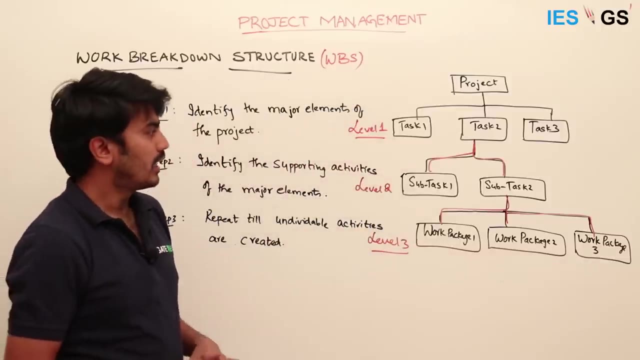 and we will be repeating the same process for the next two activities. so we will be repeating this, breaking down the task at each of this level till we each a level where each of this work package can be, each of this activity can be assigned to an independent person and which can be man manageable and which a 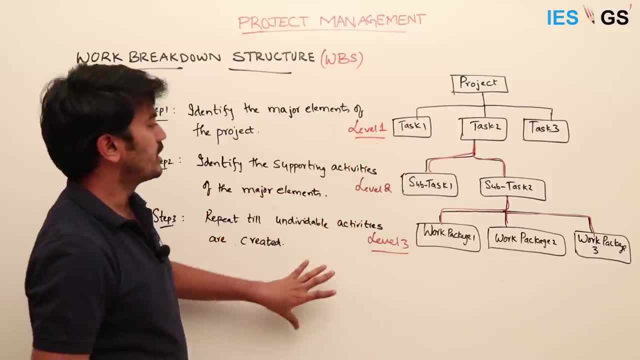 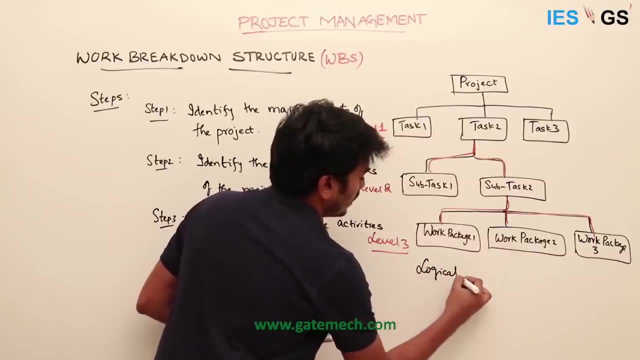 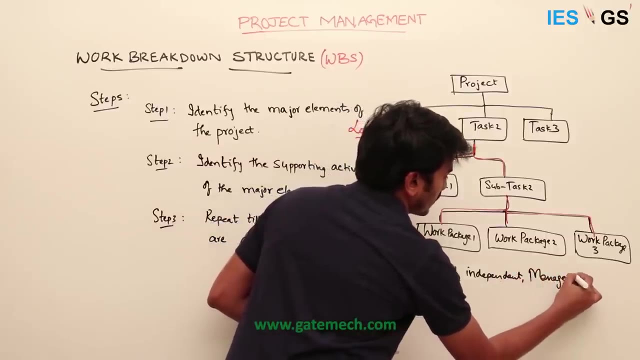 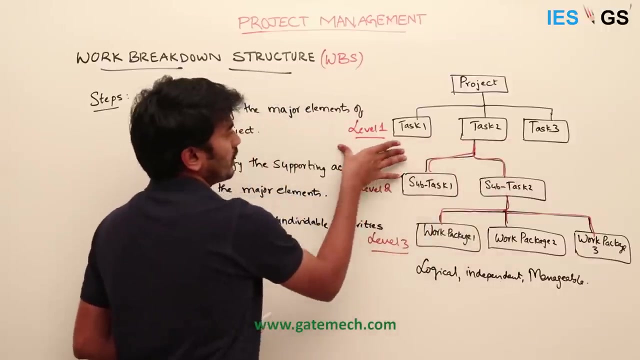 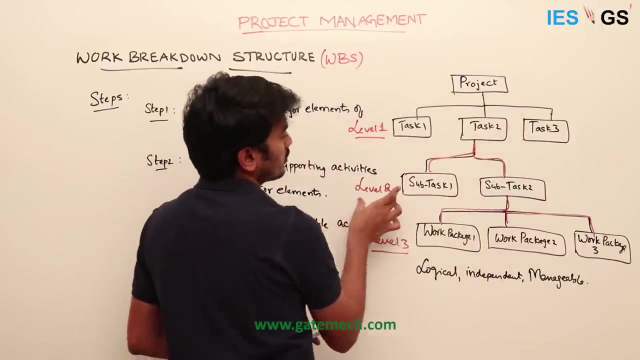 which is logical. so this process is repeated until we get the activities richard, independent and then manageable, okay, and then you can see at every level. so level 1, these three tasks- task 1, task 2, task 3- will form project, as well as at level 2 also all the 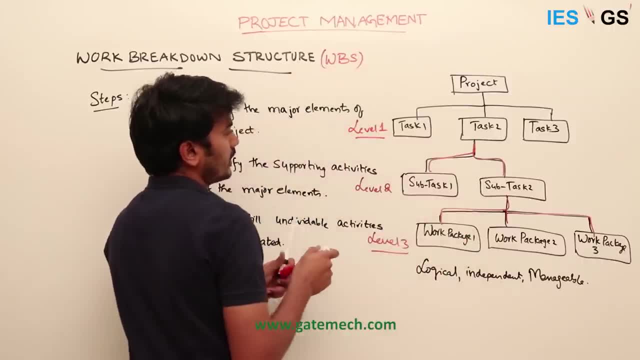 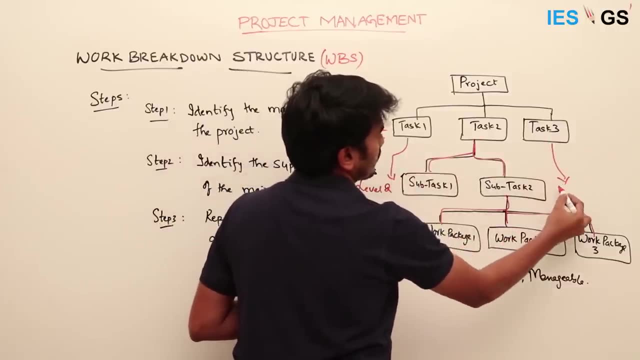 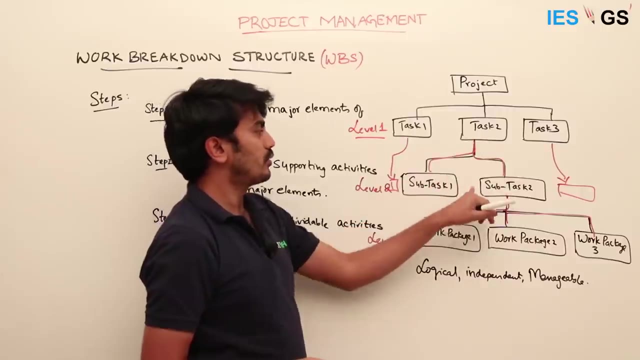 tasks that are there, so I didn't highlight this like task 1 will also be having some items, some activities. task 3 will also be having some activities at level 2, so for the illustration I took only this: task 2 activities. so at every level when 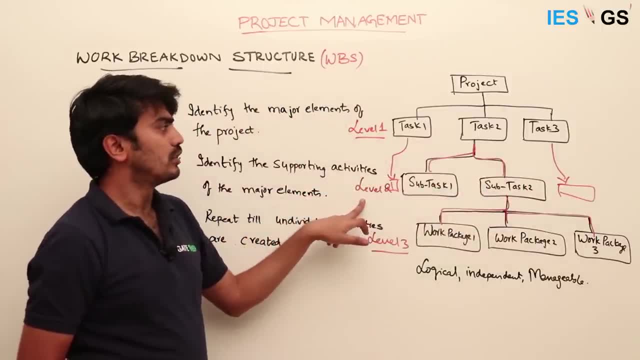 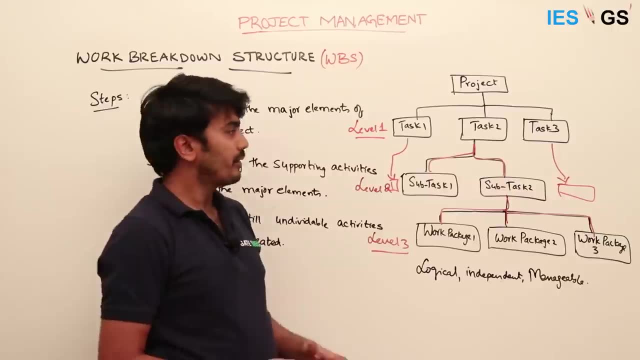 you sum up all the activities at that level, say, at level 2, they will form the complete project. similarly, at level 3, they will form the complete project. okay, so you can see that we are following a top-down approach, that we are breaking the project into three stages. so we are following a top-down approach, that we are 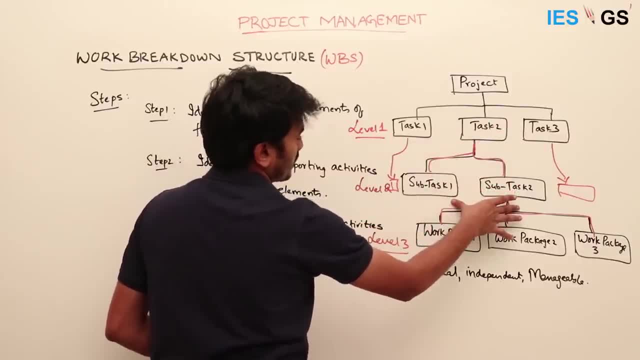 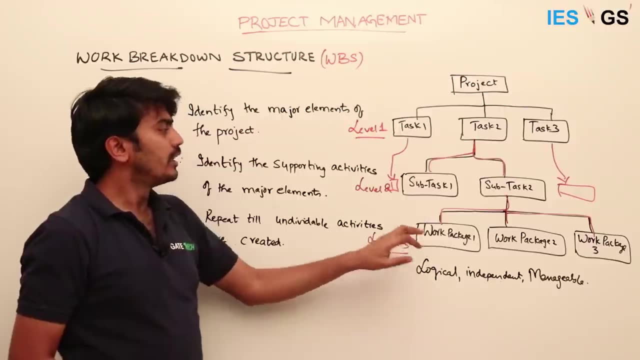 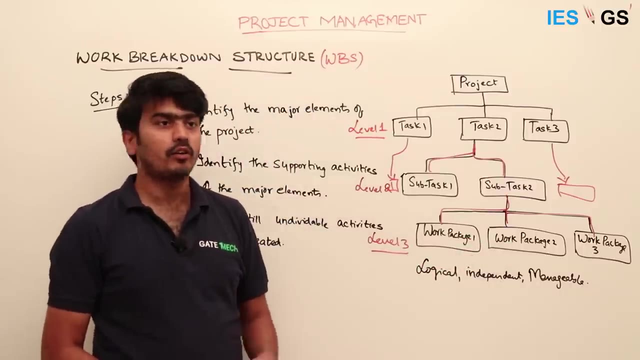 breaking the project into three stages. so we are following a top-down approach, that we are task, and then breaking them again into sub tasks. so so work breakdown structure. this technique follows a top-down approach and then it will find out the detail level work packages, based on which we can estimate the time and cost. 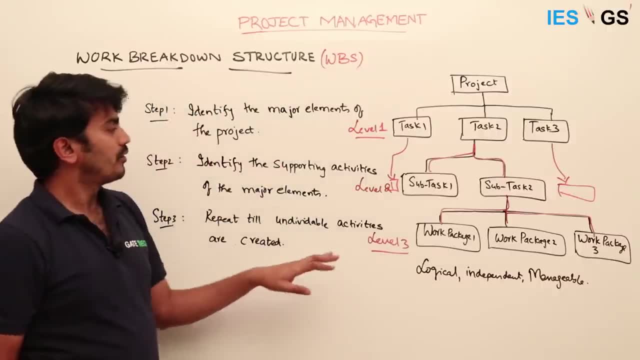 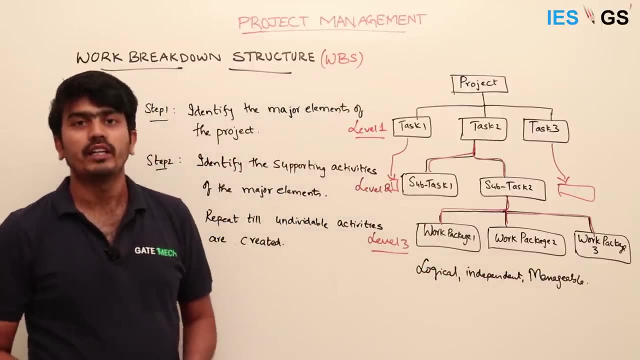 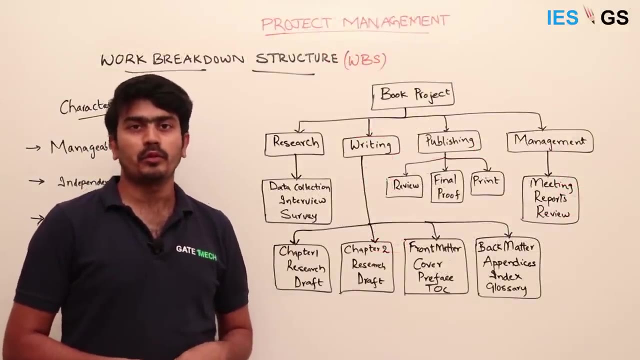 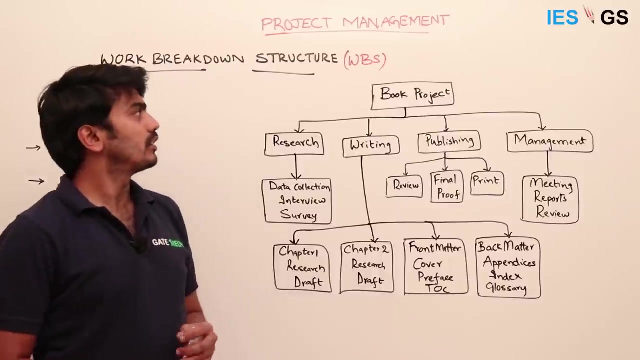 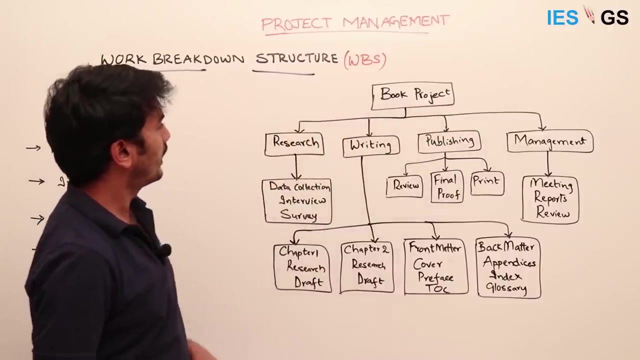 of each activity. so we will discuss what this work breakdown structure finally gives us as an output. Now let us see an example on book project: how it how work breakdown structure is used in order to find out the activities of a book project. So you can see in the picture, book project is at the top and it consists of the major 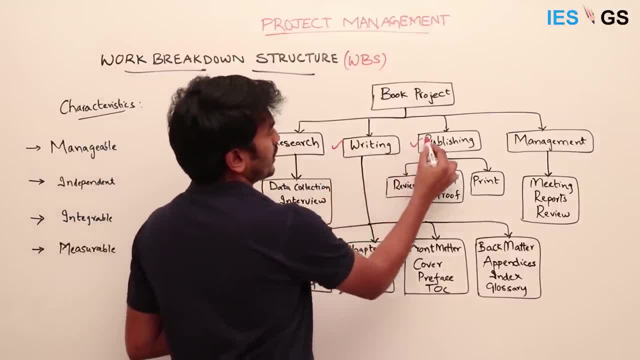 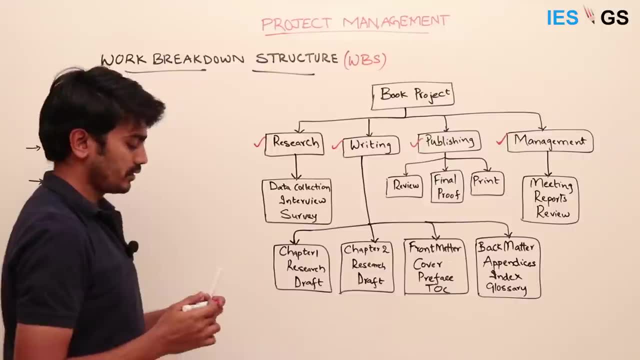 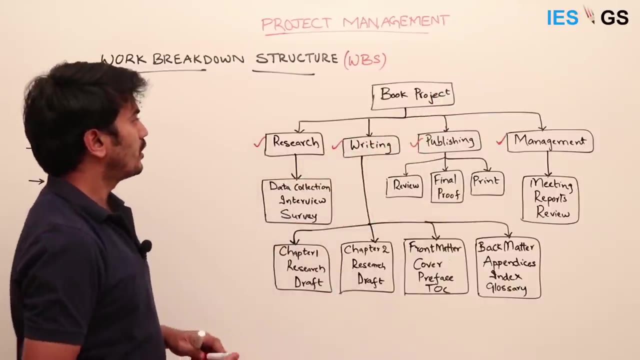 elements, that is, the research, the writing, publishing and management. So these are the major elements that are to be looked into under a book project. So in order to planning, writing and publishing a book- that is that is a book project objective. So in order to do that, so they will be doing some research and then they will be doing 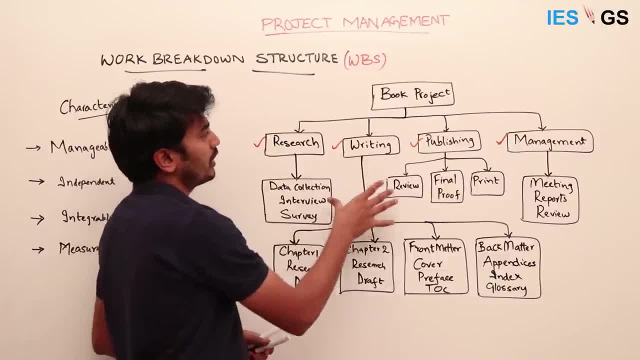 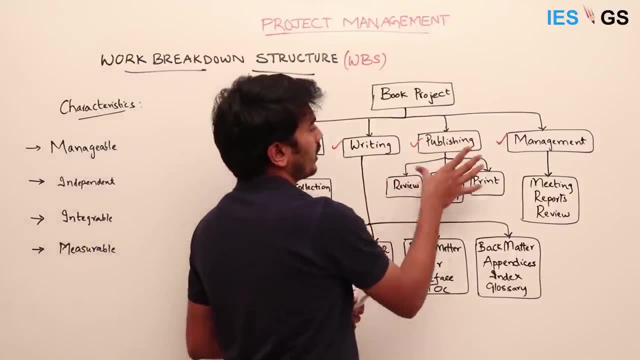 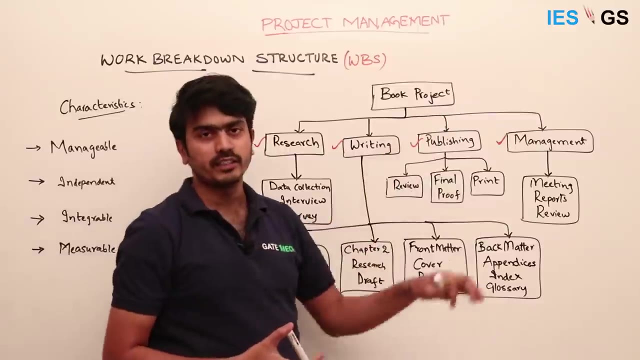 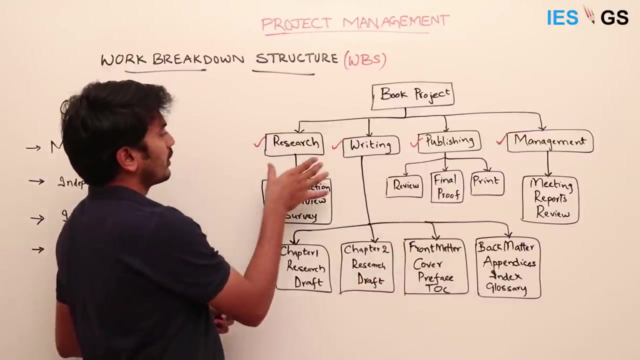 some writing the content of the actual book and then the publishing part, So who will be printing, how many copies we need to print, and then proofing all those things, And then the managing that the contents are, reviewing the book contents, etc. So these are the four major elements in which they are divided, which are, you can say, largely. 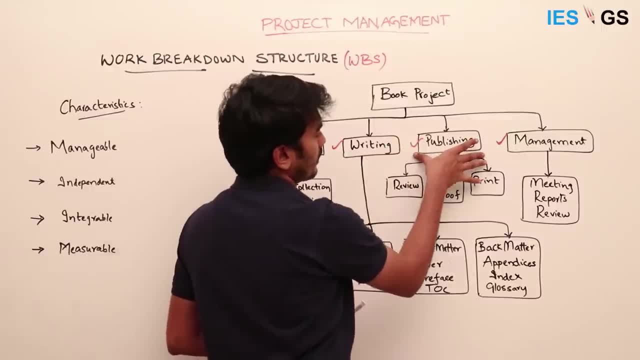 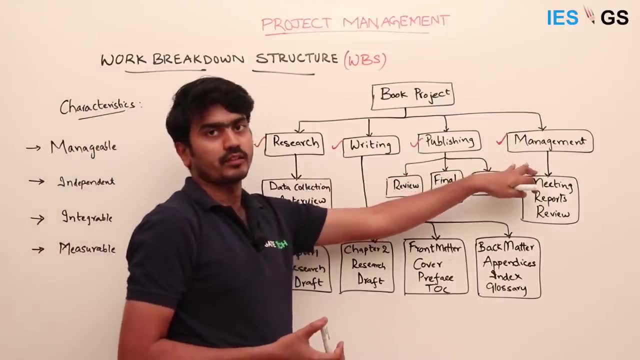 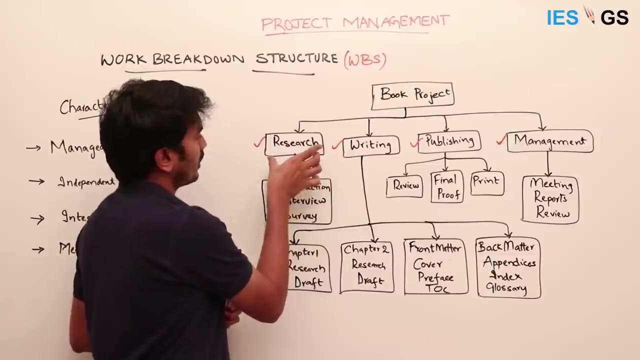 independent. So once the writing is done and then the publishing will happen after the management review happens. So they are managed separately with different stakeholders involved, and then the next level is to break down, Break down this part into details, what research actually means. it is basically consists of: 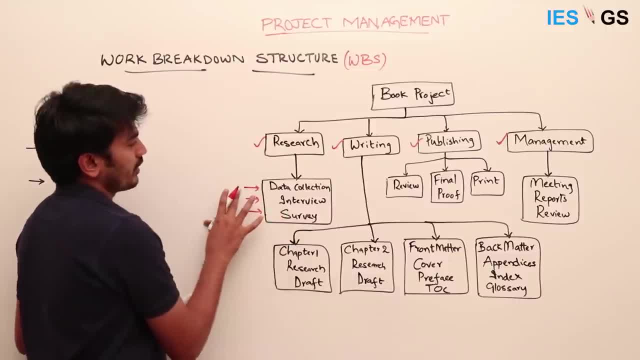 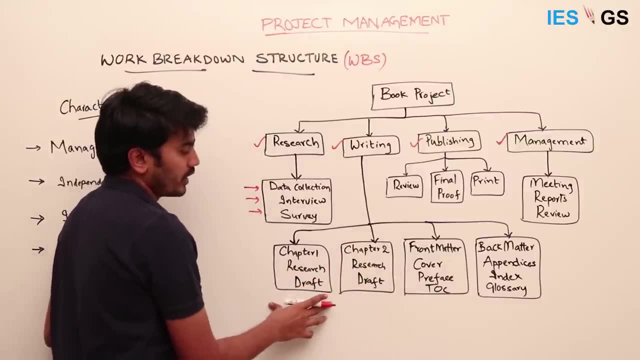 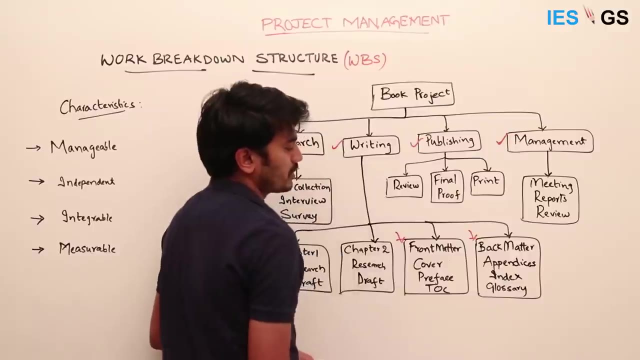 the data collection, interviews and surveys, etc. And then comes to the writing, breaking down the writing chapter wise, the research required and the initial drafts of these, each chapter. and what is the front page looks like? how is the back page looks like? what are details will be there in the cover preface. 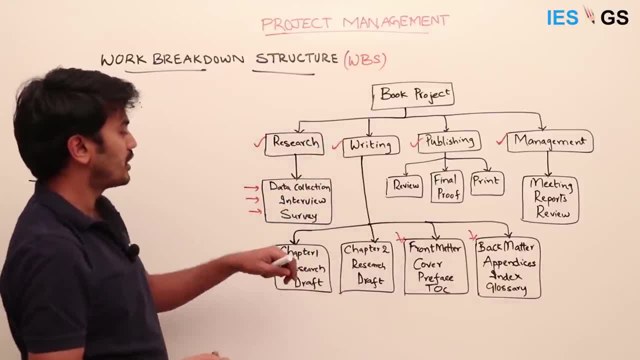 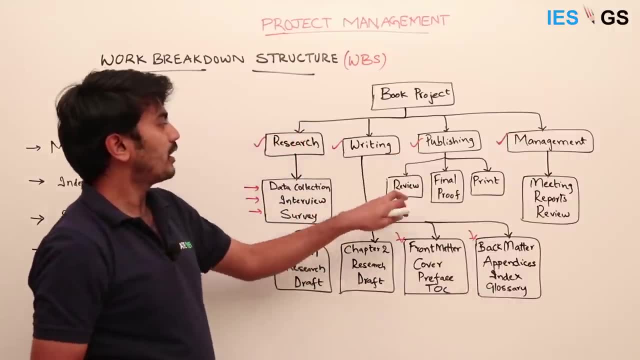 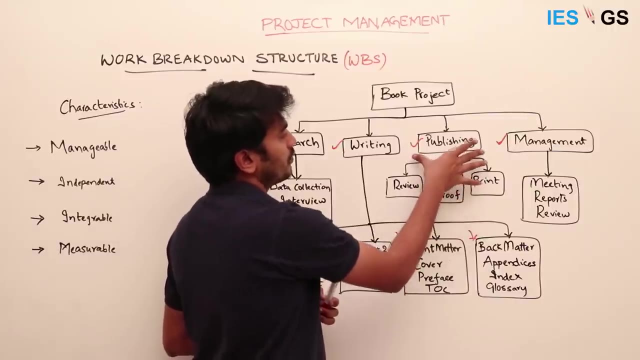 So these are the details of the actual contents of the book, which are divided into chapter wise and front related contents and back related contents, And then the publishing part will be break down into reviews, final proofs. So this is the next level of the sub components of publishing. similarly, sub components of 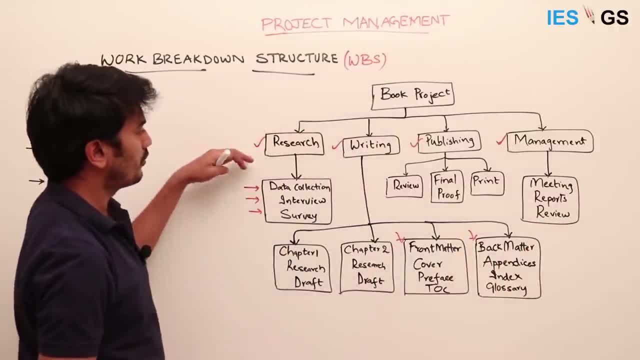 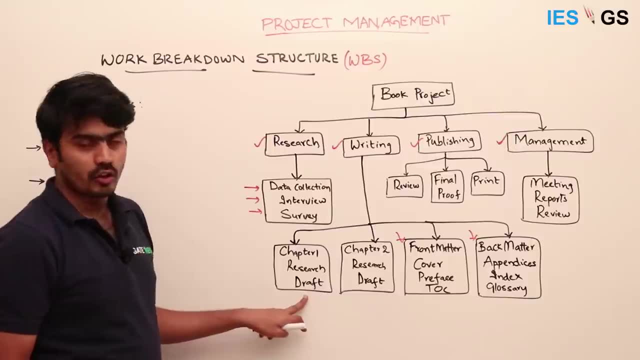 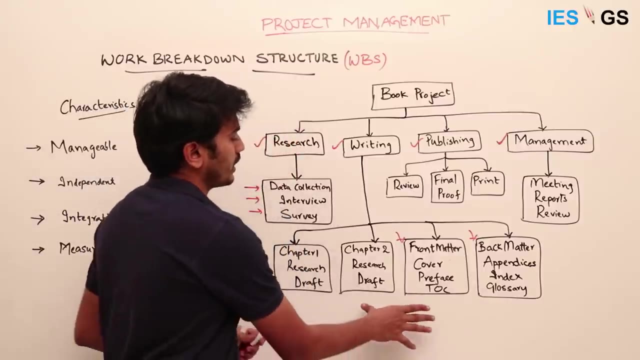 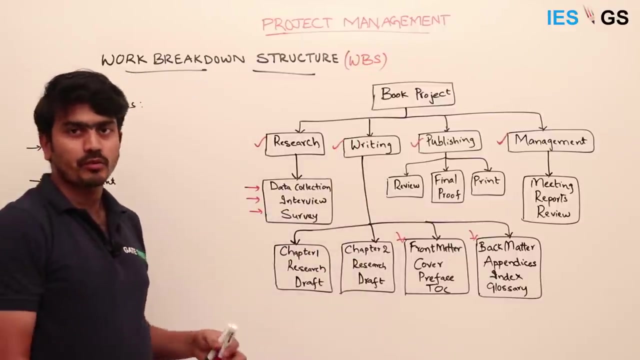 management. So this is basically a top down approach where we are finding out the detail activities that are to be performed, Which are, Okay, Logical, independent and manageable, okay, So, and then these will get combined and become the final book project. So the number of levels will change based on the project, based on the nature of the 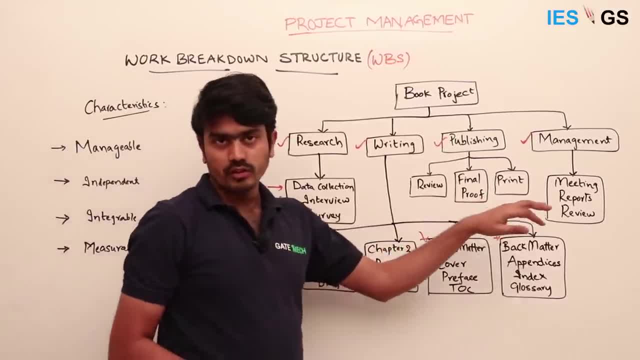 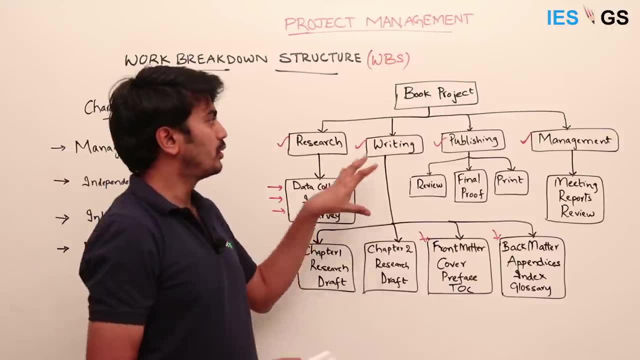 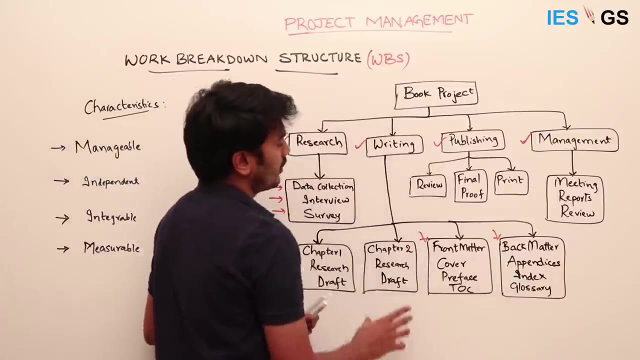 project and the number of activities at each level also will change based on the project, So that are based on the experience or the expertise of the people involved who is developing this work breakdown structure. So once we have this detail level activities, we will estimate what is the time and effort. 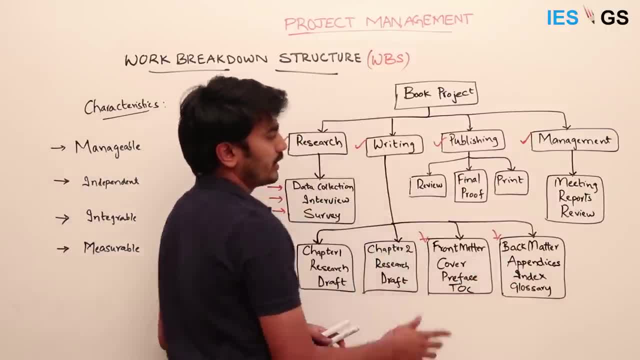 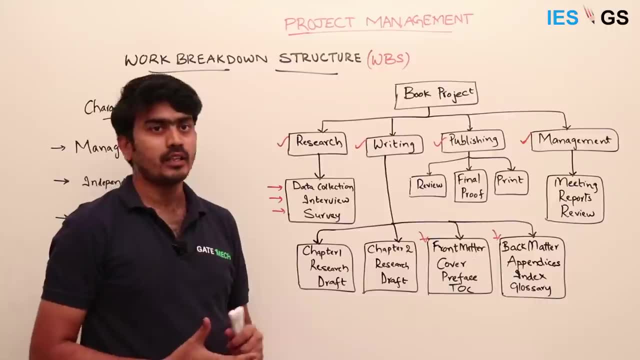 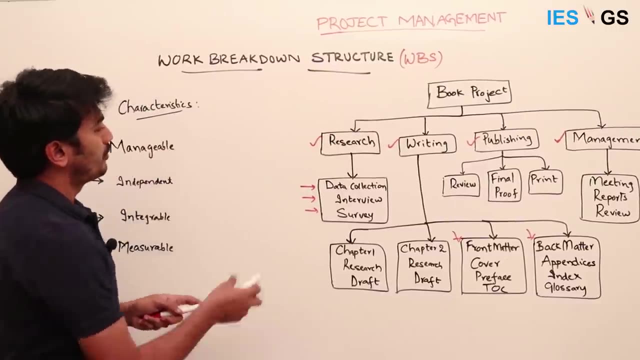 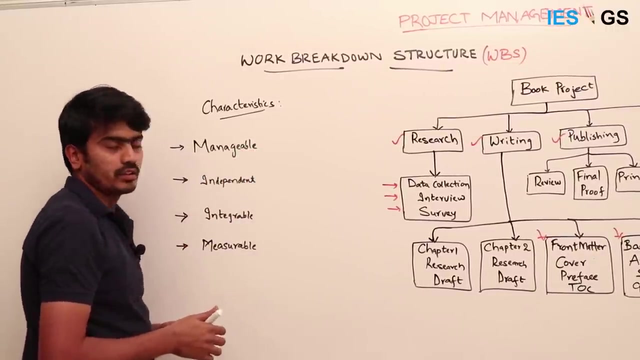 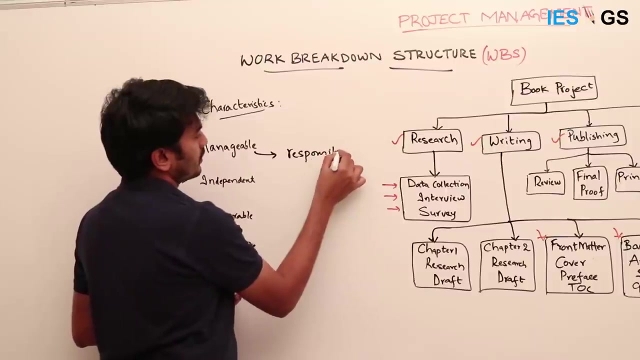 required of each of these activities and then combine to arrive at the total project cost and duration. Okay, so checking the characteristics of the work breakdown structure while performing this activity we need we should be looking at the activities that they should be managed So it can be assigned as a single responsibility, okay, and then the activity should be independent. 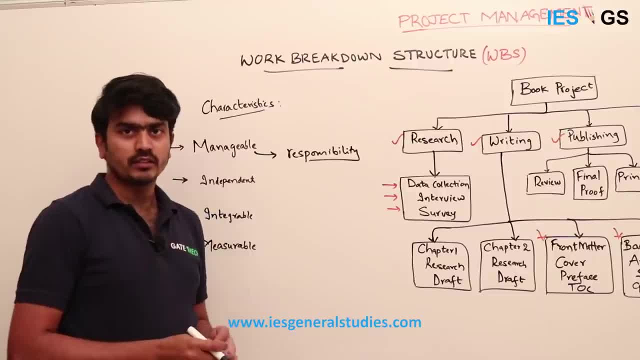 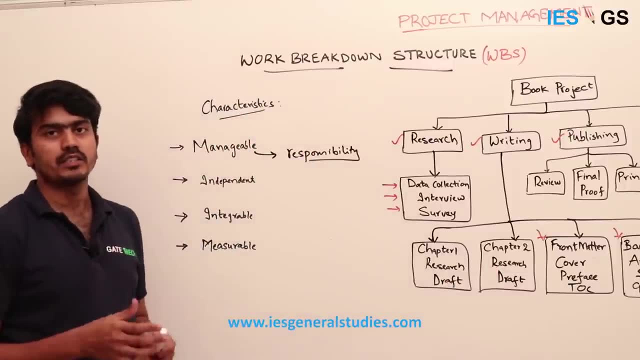 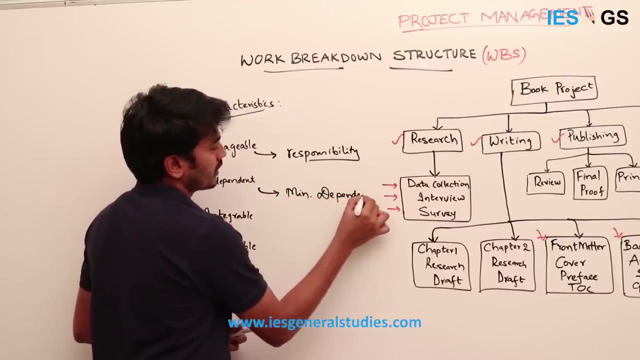 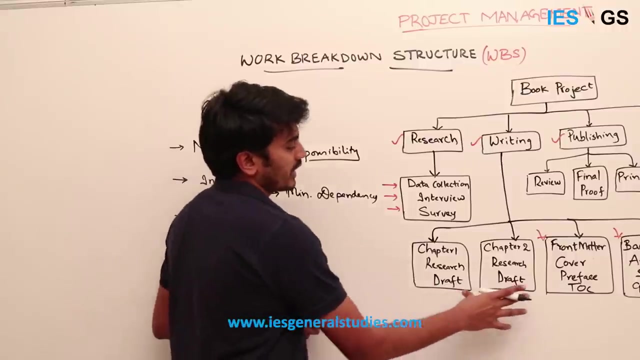 the there should be minimal dependency on other things. So there, so that it can be executed separately without any, without, without, in the sense, minimum dependency, that is, minimum dependency on other things, Okay, And then it should be integrable in the sense. so these activities, when performed individually. 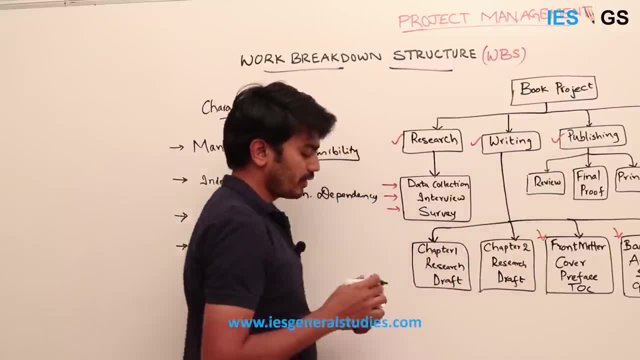 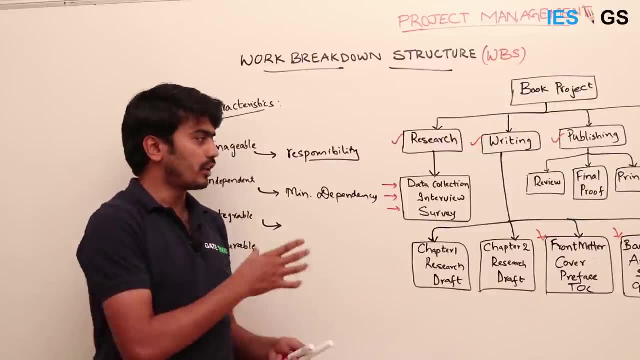 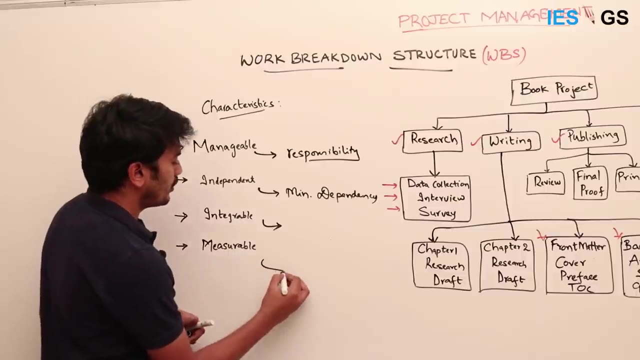 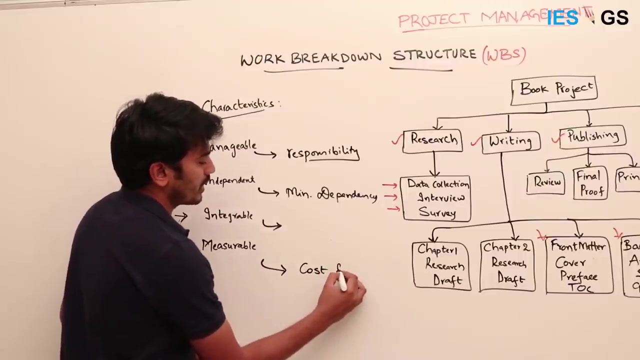 should get integrated easily so that we will arrive at the final project. Okay, so it is more relevant in case of software products where one component should be compatible with the other component that is developed independently, and then it should be measurable In the sense we can. it should be easily estimated in terms of cost and time required, and then